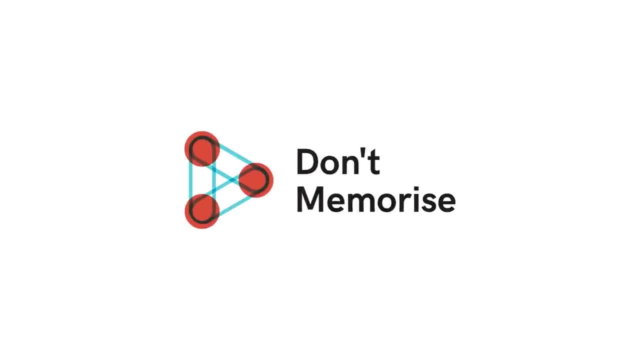 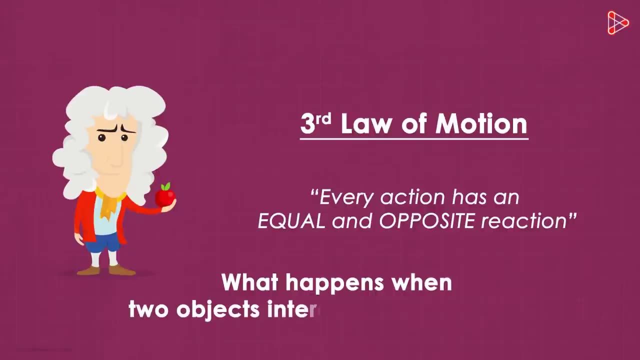 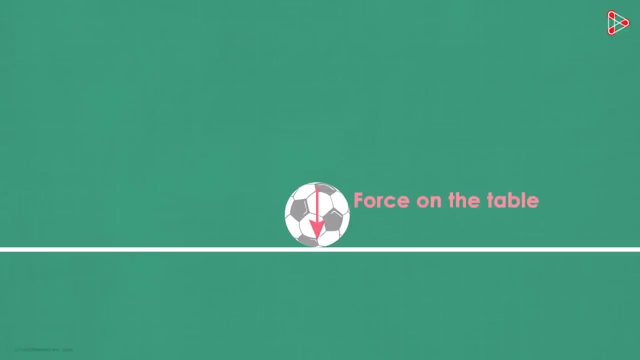 The only question you need to ask yourself while studying the third law is: What happens when two objects interact with each other? What happens when you place an object on the table? The object exerts a force on the table and the subject exerts an upward force on the object. 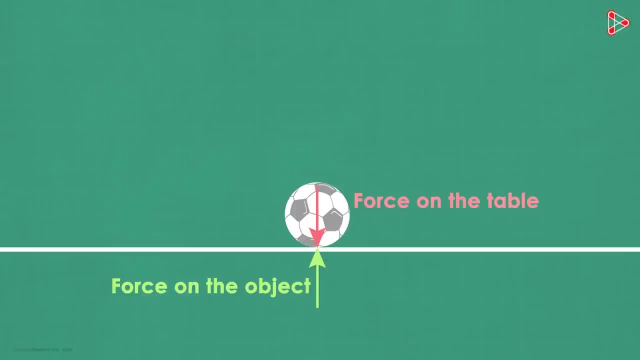 There are two forces that result from this interaction: A force on the table and a force on the object. The magnitudes of the two forces are the same, but the directions are opposite. These forces are called as action and reaction forces. The force exerted by the object on the table was an action force. 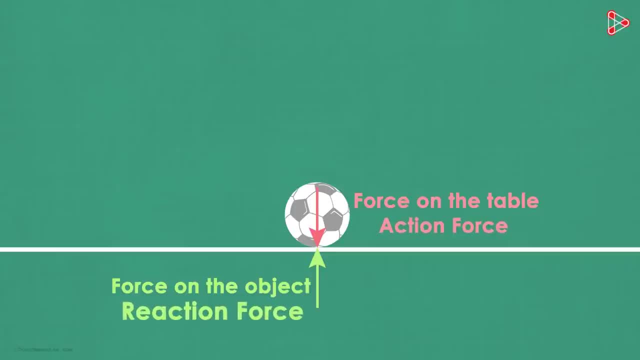 and the force exerted by the table on the object is the reaction force. What we saw here is nothing but a display of the Newton's third law of motion. Every action has an equal and opposite reaction. That's how simple the third law of motion is. 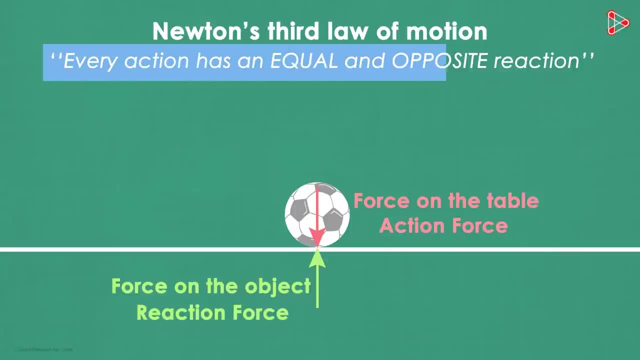 Every action has an equal and opposite reaction. It means that when two objects interact, there is a force on each object. The magnitude of force on the first object equals the magnitude of force on the second one. And what about the direction? The direction of force on the first object is opposite to the direction of force on the second one. 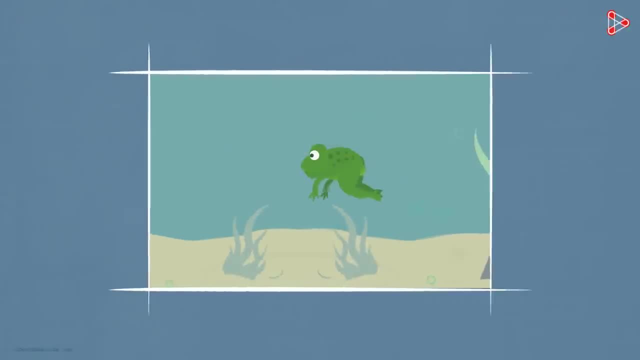 Let's talk about more examples. While a frog is swimming, it pushes the water back And the water pushes its body forward. Now let me ask you a question. Say a bird is flying upwards. Will the Newton's third law apply here? 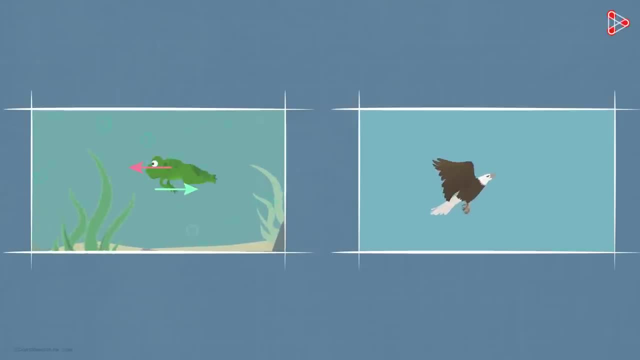 Sometimes the third law is not so obvious. You'd probably say that the bird is the only object here and there's no second object, But that's not correct. The wings of the bird push the air downwards and the air pushes the bird upwards. 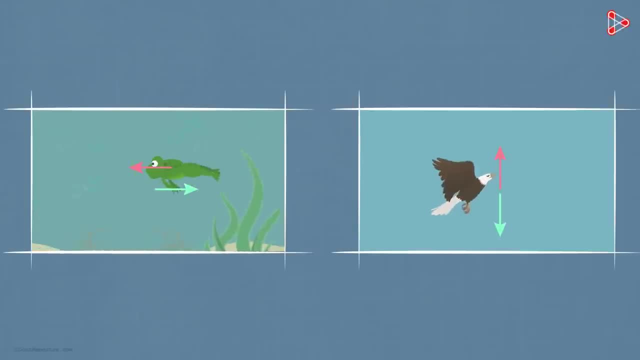 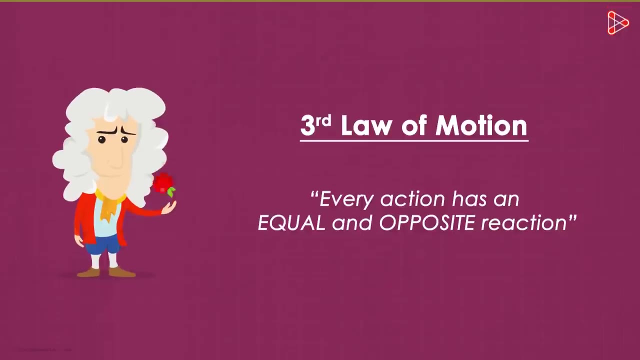 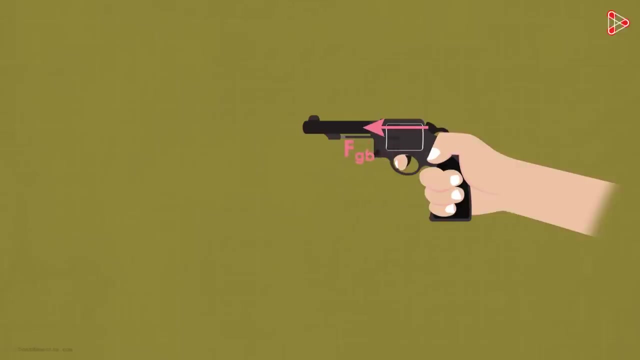 Action and reaction forces make it possible for birds to fly. We take one last example to understand something very interesting about the third law. What happens when a gun is fired? You're right. It exerts a forward force on the bullet And the bullet exerts an equal and opposite reaction force on the gun.